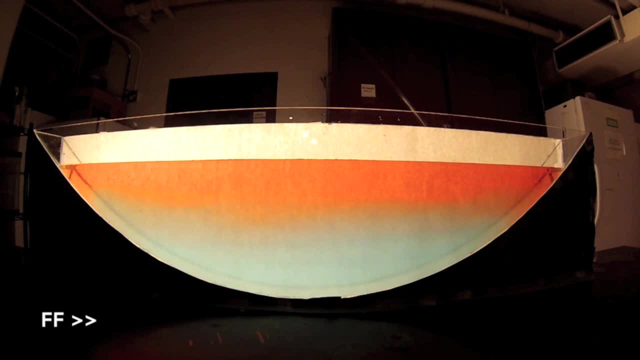 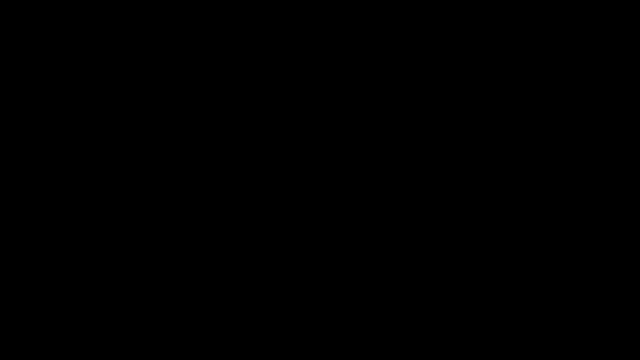 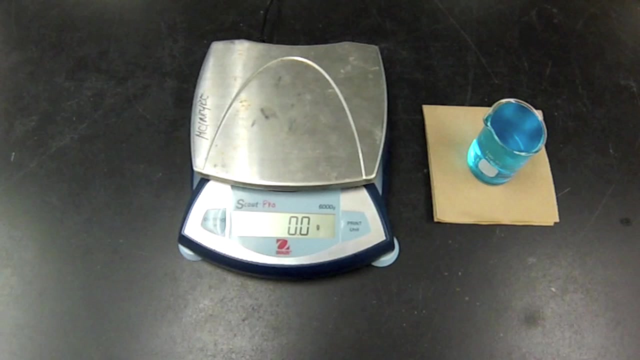 Once again, the warm water settles out on top. What's going on? To answer that, we need to take a look at the physical principle driving the whole show: density. Density is the amount of stuff in a given volume. In our case, that stuff is water, and 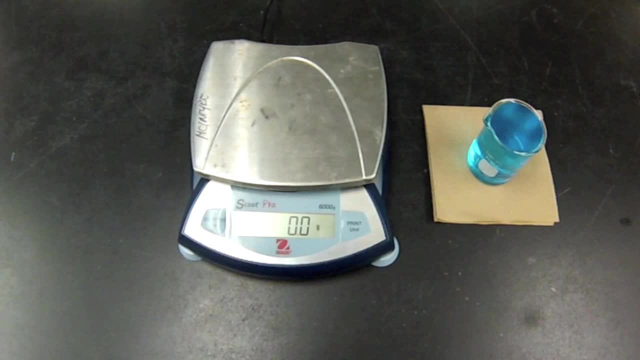 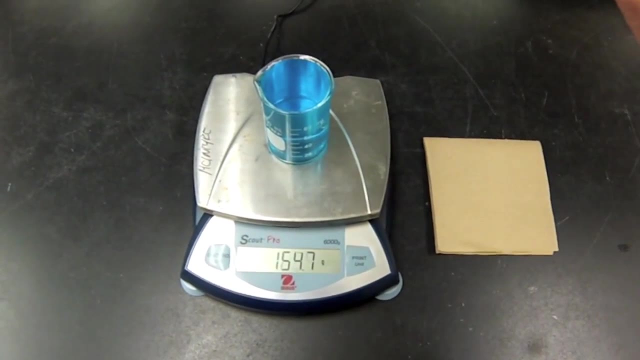 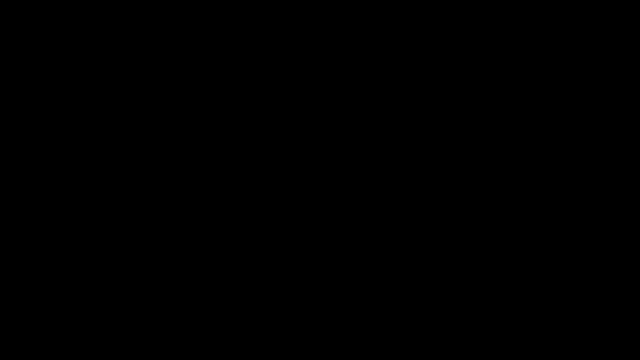 that volume is this glass beaker. This beaker is filled to the brim with our cold water. Let's see how much. its weight is 166.2 grams. Now we've emptied the cold water and refilled the beaker with the warm water. The warm water weighs in however much water is. Monica's weight is 36.2 pounds. And the warm water weighs in everything, Because this beaker itself is stored in this trash can inside the corner. So this drank vice has the high density- greaterächly 100. glaube justice to the solid matter. Density is the amount of stuff in a given volume. In our case, that stuff is water. In that volume is this glass beaker. This beaker is filled to the brim with our cold water. Let see how much it weighs. 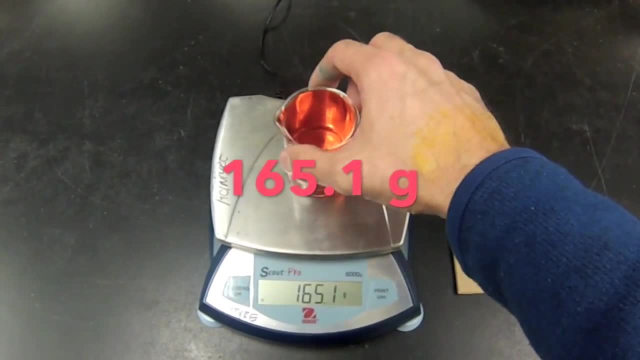 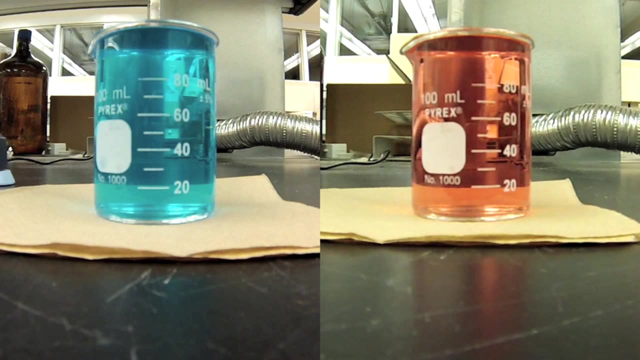 water weighs in at 165.1 grams, a little bit less than the cold water. We can calculate the density of these two samples by dividing the mass by the volume. First, we need to correct our previous measurement by subtracting out the mass of the empty beaker. This gives us 116.2 grams for the. 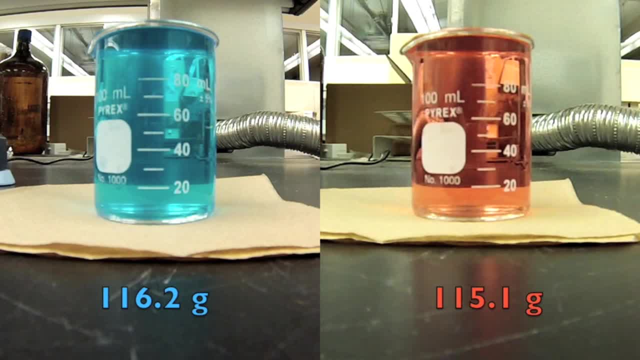 cold water and 115.1 grams for the warm water. Now we divide by the volume of the beaker to get a cold water density of 1.00 grams per milliliter and a warm water density of 0.99 grams per. 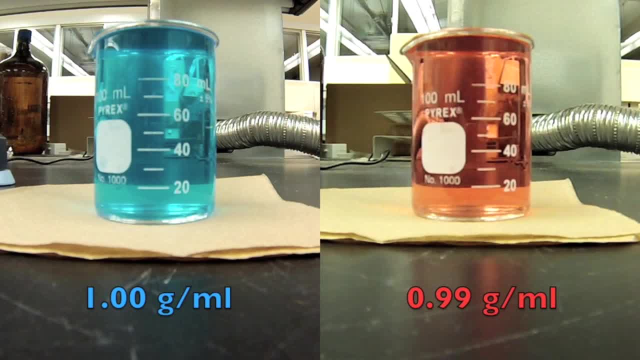 milliliter. In reality, it's a very small difference, but that small difference has a big impact. It allows the warm water to essentially float on top of the cold water and it keeps the two layers from mixing together. So what affects the temperature and, in turn, the density of the 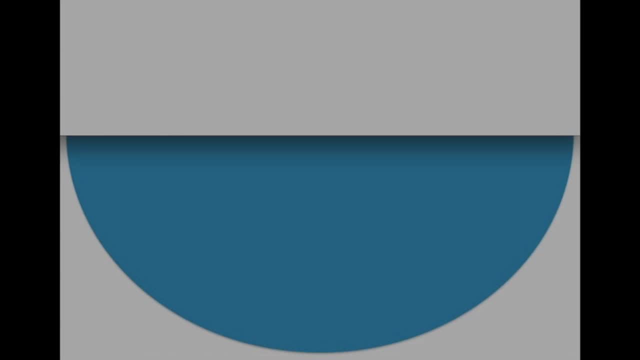 water in the lake. You might think the temperature of the air surrounding the lake is the answer, but really the biggest impact comes from the sun. As sunlight enters a lake, it warms the surface water, making it less dense and lighter As the surface water begins to float. 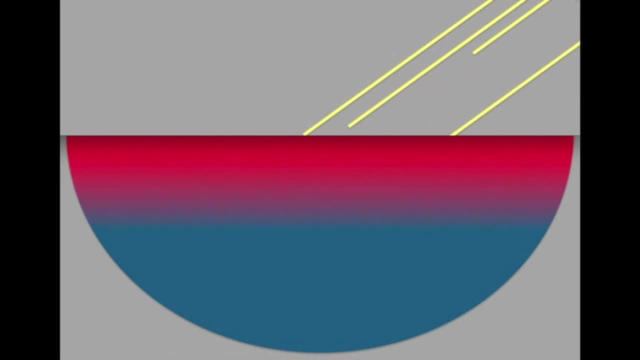 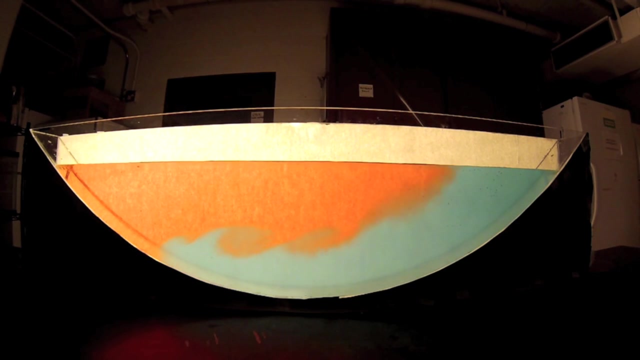 on the cold water below, a transition zone forms where it changes from warm to cold very quickly. We call that the thermocline. Remember, thermal stratification in lakes is as ordinary as the changing of the seasons and in fact it does change with the seasons.